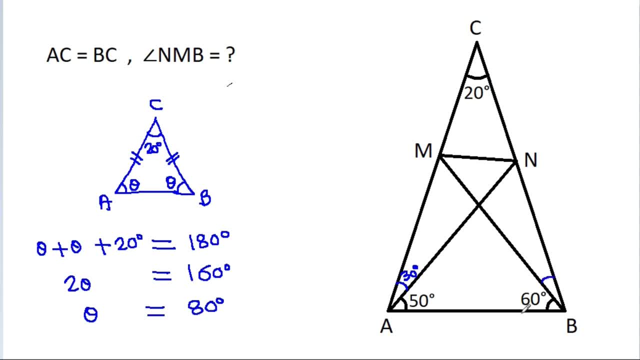 And this angle will be 80 minus 60, that will be 20 degree. And now in ABN this angle is 50 degree, this angle is 80 degree And this angle, suppose theta. So 50 degree plus theta plus 80 degree. 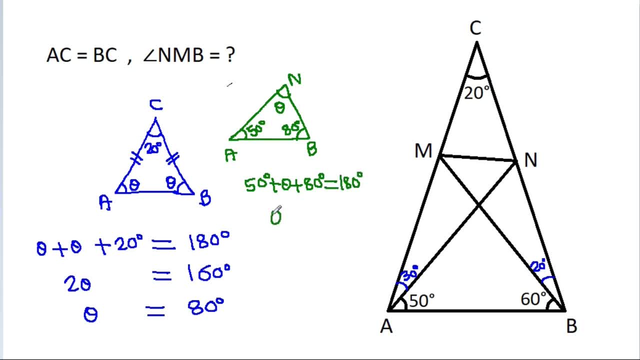 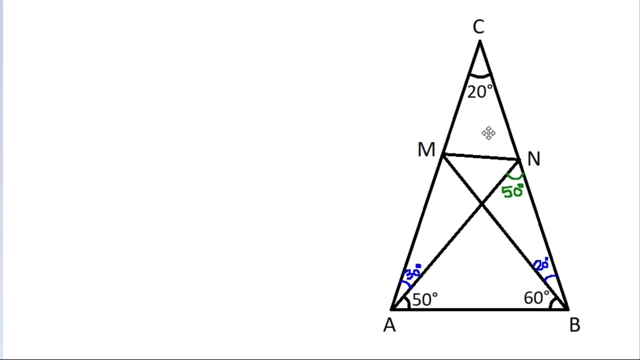 it will be equal to 180 degree. So theta will be equal to 50 degree. This angle it will be 50 degree And and this should be 30 degree Now in ABN, this angle is 50 degree. this angle is 50 degree. 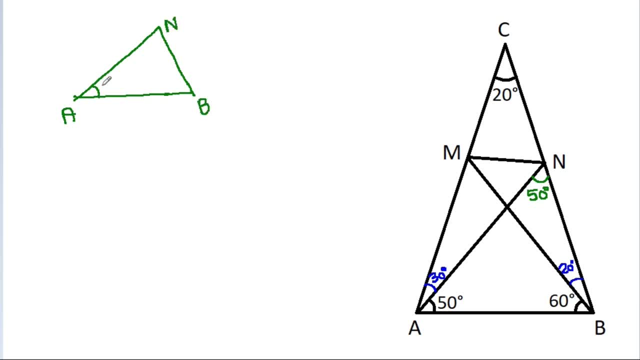 Now in ABN, this angle is 50 degree. this angle is 50 degree, So AB will be equal to bN. Our angle is 50 degree, so our angle is 50–50.. If this angle be 20 degree, then also this angle will be equal to 50 degree. 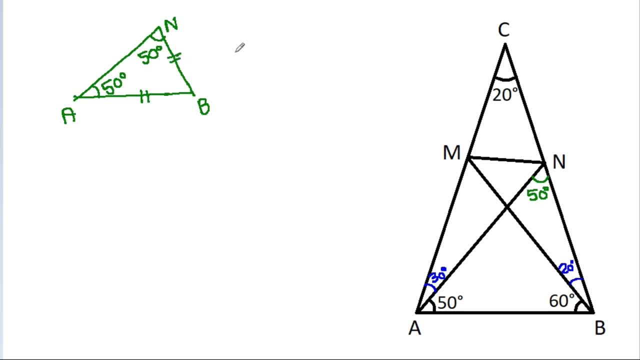 Thereby we have to work on line ABN. the tempo is 150 degrees, So AB will be equal to bN, The karate 같이ний angle. This is angle for 80 degree. So close your eyes so that you notice when you consider the angle. 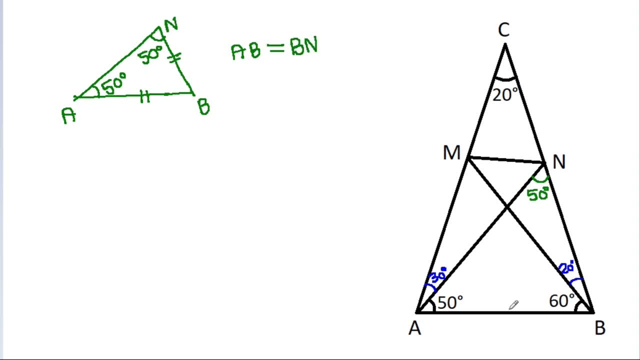 AB will be equal to 50- explained. Yes, that's right ~~. AB and BN will be equal and in triangle, AMB it is AMB, this angle is 80 degree, this angle is 60 degree, this angle suppose theta. so 80 degree plus 60 degree plus theta, it will. 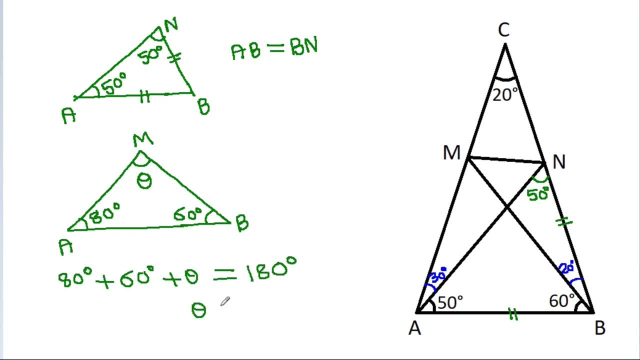 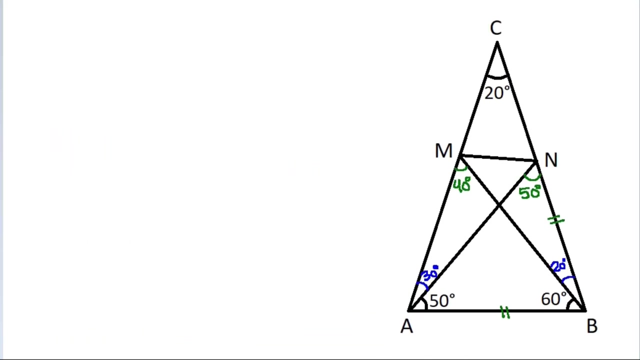 be equal to 180 degree, so theta will be equal to 40 degree. this angle will be 40 degree, and, and, and, and, And. and. Now, if we draw BD, suppose this point is D, such that AB is equal to BD. it is our construction. 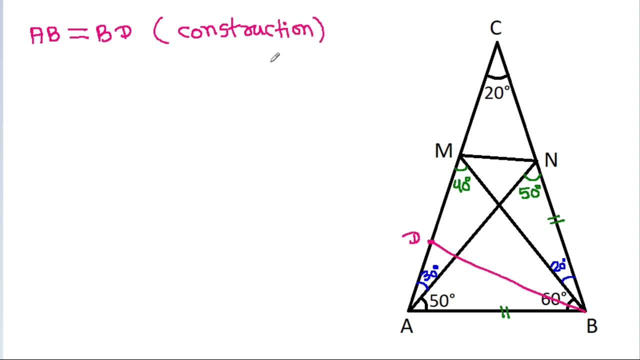 Then in ABD it is ABD, this angle is 80 degree and AB is equal to BD. so this angle will be also 80 degree And this angle suppose theta. so 80 degree plus 80 degree minus theta will be equal to. 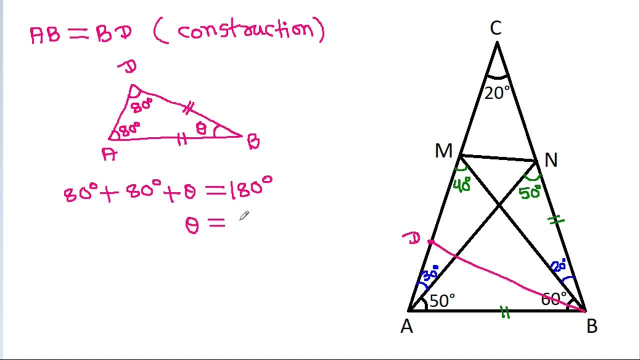 180 degree, so theta will be equal to 20 degree. This angle is 80 degree and this angle is 20 degree, So this angle will be 60 minus 20, that will be 40 degree. and now in BDM, it is BDM this. 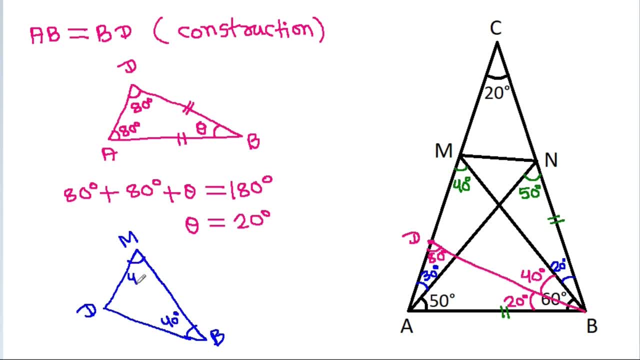 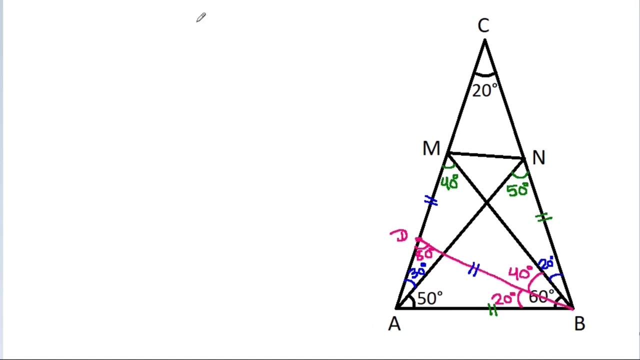 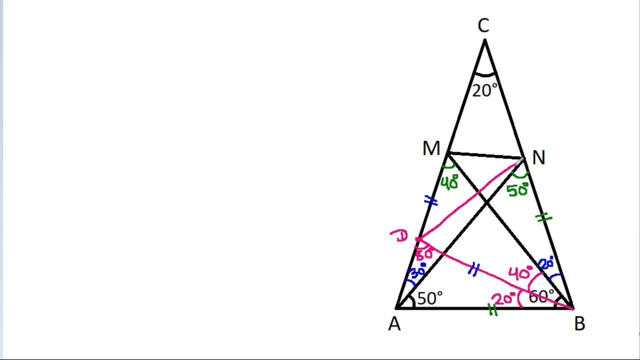 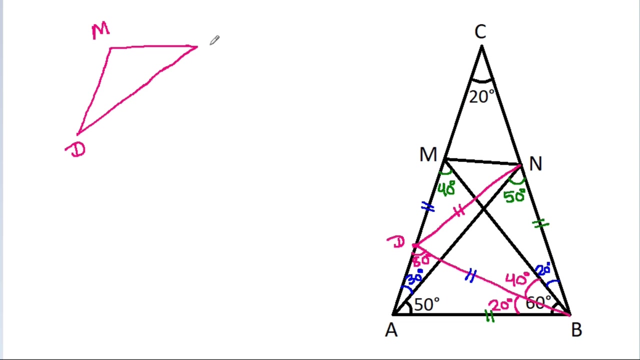 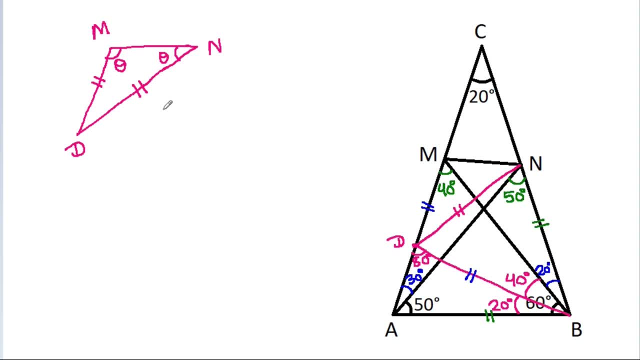 So these two angles will be equal, and here dnb it is equilateral, so this angle will be 60 degree, this angle will be 60 degree. And this point is d, This angle is 80 degree, this angle is 60 degree, so this angle will be 40 degree. 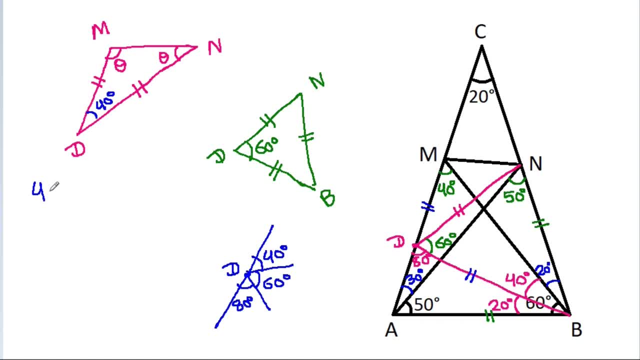 This angle is 40 degree, so 40 degree plus theta. plus theta it will be equal to 180 degree. and 2 theta is equal to 140 degree, So theta will be equal to 180 degree. And this angle is 40 degree, so this angle will be 30 degree.